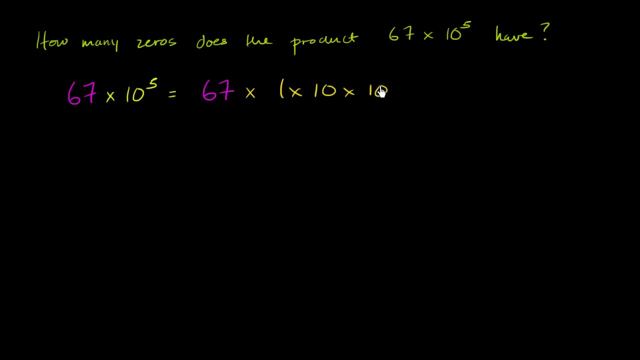 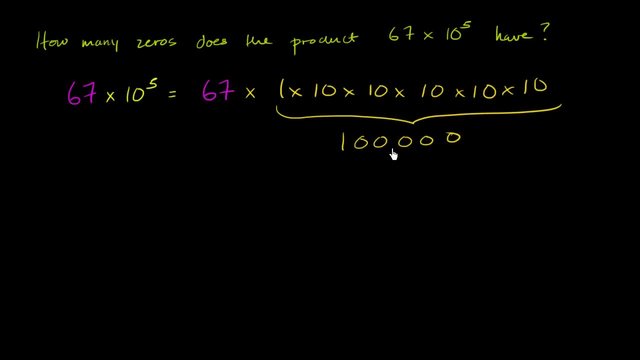 One, two, three, four, five, So it's going to be 100,000.. So there's a couple of ways to think about it. If you're looking at just this product right over here, you could say: well, 67 times 1 is just going to be 67.. 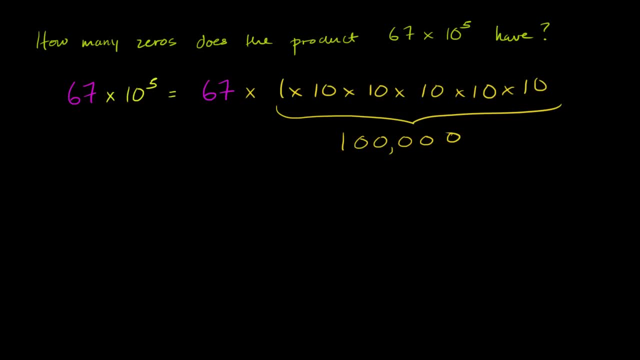 And then every time you multiply by 10, you're going to add another 0. So you could say: well, this is just going to be 67. And we're going to be multiplying by 10 five times. So we're going to add five 0's here. 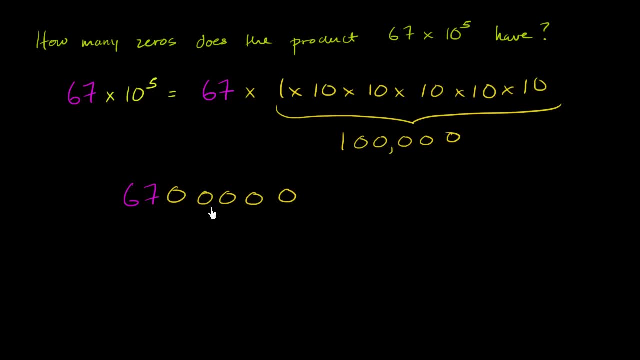 One, two, three, four, five, And so this would come to 6,700,000.. Another way you could think about it, this is the same thing. It's the same thing as 67 times 100,000. 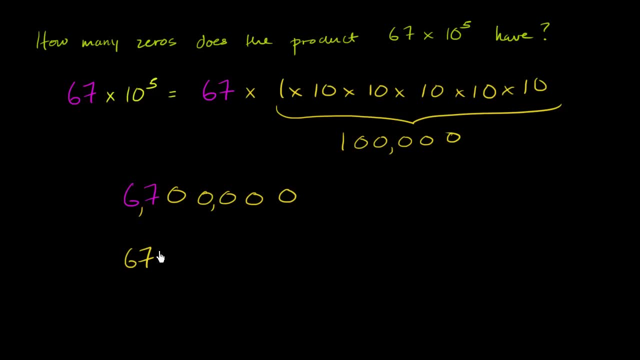 So it's going to be 67.. And then we have five 0's here. So once again, one, two, three, four, five, You get the exact same value. Let's do another one: How many 0's does the quotient 5,700,000 divided? 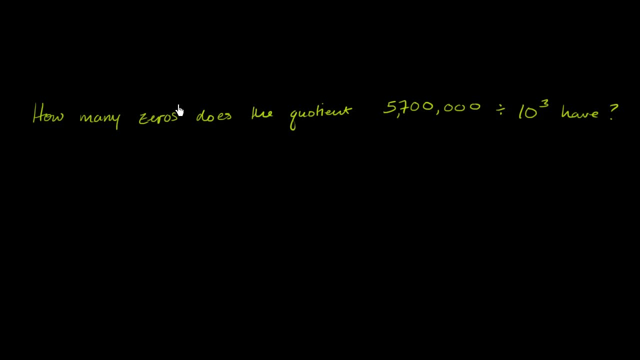 by 10 to the third power. have Well, 10 to the third power. we already know: 10 to the third power. that's the same thing as 1 times 10, times 10, times 10.. Which is the same thing as 1,000.. 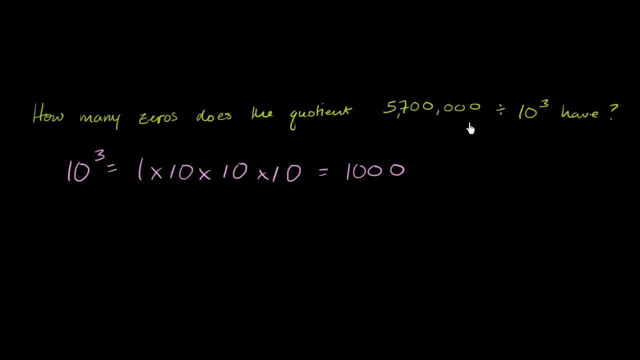 And so if we're dividing by that, that's the same thing. So another way of writing this expression right over here: So 5,700,000 divided by 10 to the third is the same thing, as I could write it this way: 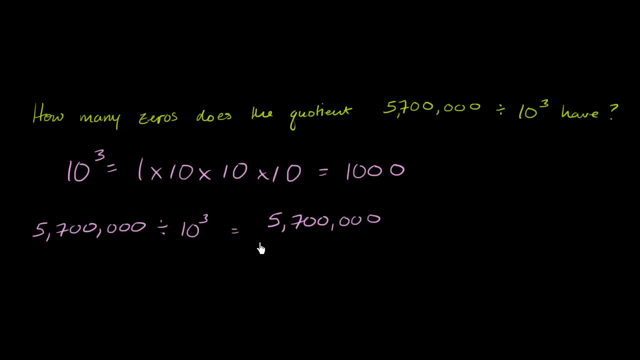 5,700,000 divided by 10 times 10, times 10.. We could put a 1 out here, but this won't really change the value, Which is equivalent to 5,700,000 divided by 1,000.. 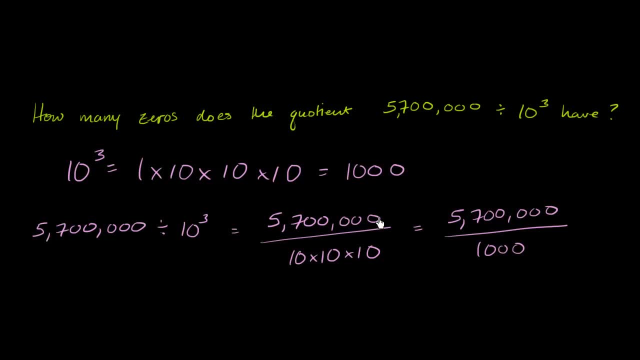 And either way you think about it, every time you divide by 10, you're going to eliminate one of these 0's. So if you divide by 10 three times, if you divide by 10 once, you're going to eliminate a 0. 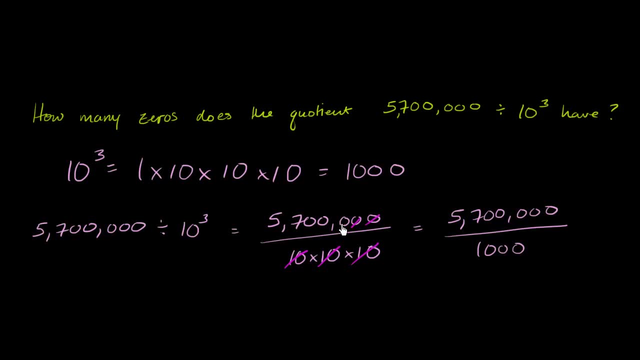 Divide by 10: again you're going to eliminate another 0.. Divide by 10: again you're going to eliminate another 0.. You're going to be left with 5,700.. Another way of thinking about it is: well, if I'm dividing by something that has three 0's. 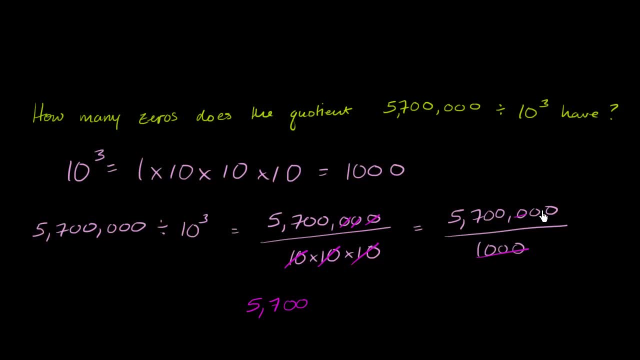 I'm going to eliminate three 0's. So if I eliminate three 0's, I eliminate three 0's. I am left with 5,700.. Now, just to be clear, I could only do this because this was 1,000. 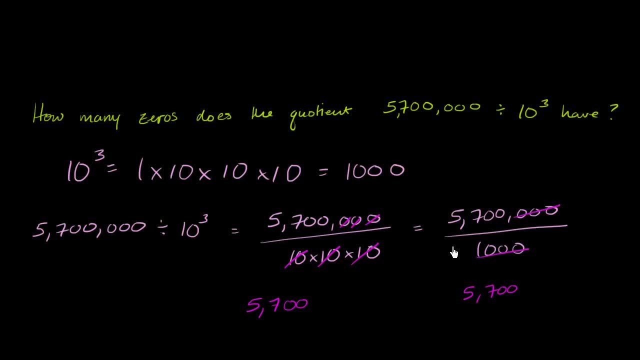 If this was like 3,000 or something, I could think of this as 3 times 1,000. And then I could only cancel out the 1,000 with these 0's, But the 3, I would then have to divide separately. 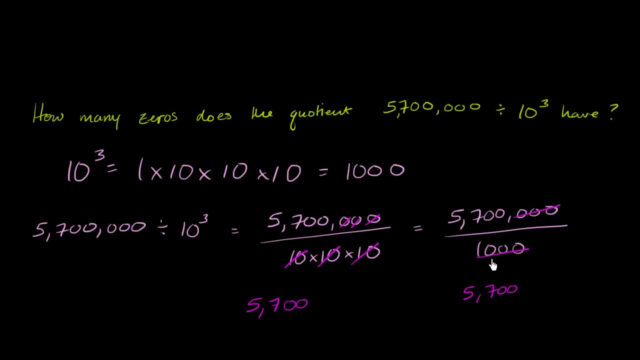 But only because I'm straight up dividing by 1,000.. I'm dividing by a power of 10.. I have three 0's here. I can cancel it out with three 0's there. Let's do another one. So I'll actually do a few. 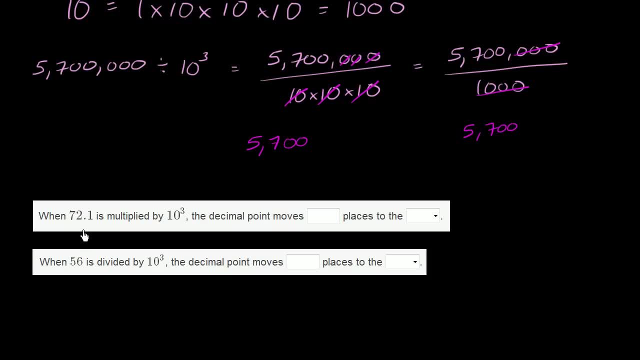 And these are the type of exact questions that you might see in the exercise. When 72.1 is multiplied by 10 to the third, the decimal point moves blank places to the blank And in the exercise you might see a drop down here. 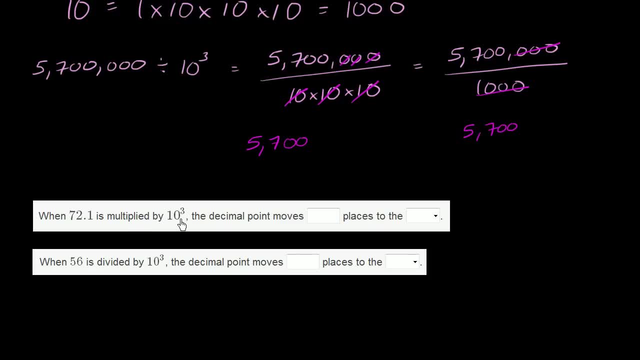 So remember, if you're multiplying by a- and this is essentially 10 to the third, as you're multiplying by 1,000, you're going to get a larger number, You're not going to get a smaller number, And so every time you multiply by 10,. 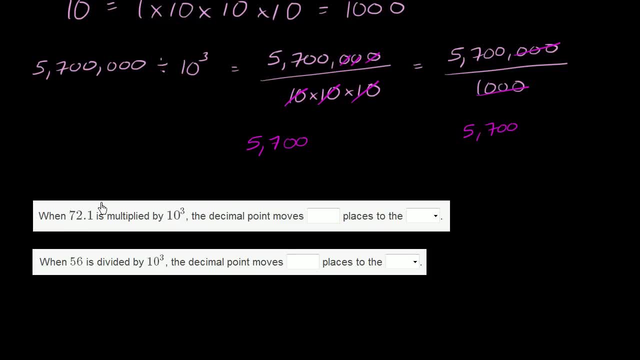 your decimal point is going to move to the right because you're getting larger, So we're going to move the decimal point. So 72.1,. if we multiplied it by 10 once, then we would move the decimal point over once. 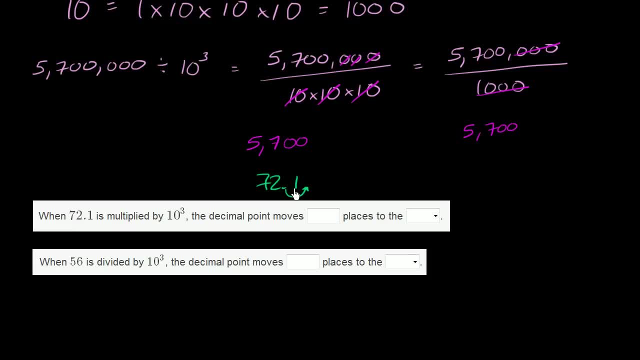 And we get 721, which makes sense. 72 times 10 is 720.. 72.1 times 10 should be 721. But if we want to multiply it by 10 three times, we're going to move the decimal place over, not just once. 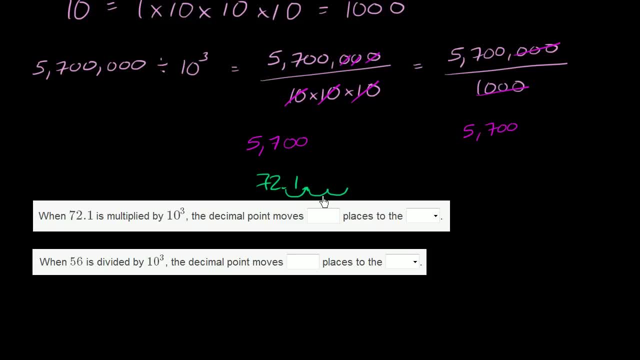 but twice and three times And you say, wait, wait, how can I move it over? There's nothing here. Well, you throw a 0 in there And so you're going to get. it's going to be equal to 72,100. 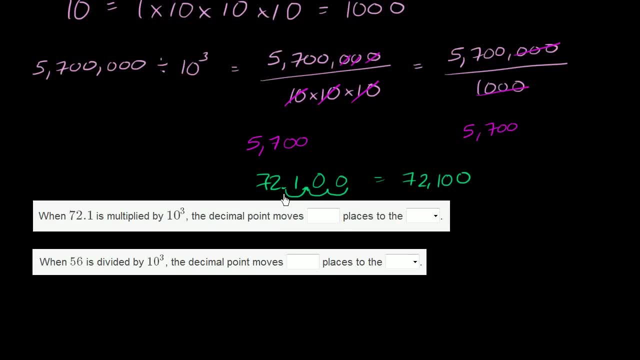 Now, they're not asking us that, They're just asking how we would do it. And we saw: the decimal point moves three places to the right And the big key here is: you're going to get a larger number when you multiply by 10, three times.